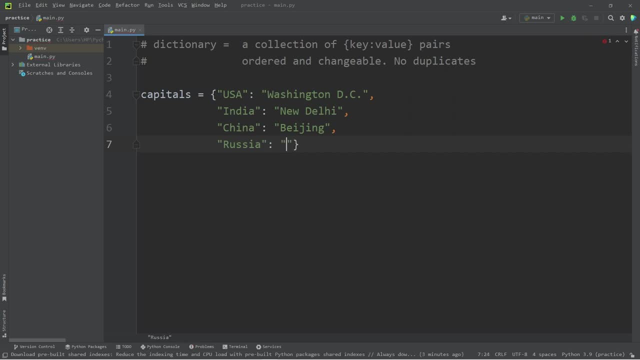 Russia, the capital is Moscow. I think that's good enough, Just as a reminder. if you would like to see all of the different attributes and methods of a dictionary, you can use the dir function: pass in your dictionary capitals, then we'll need to print this. 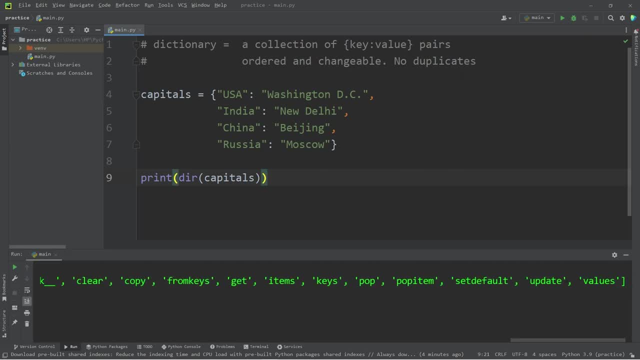 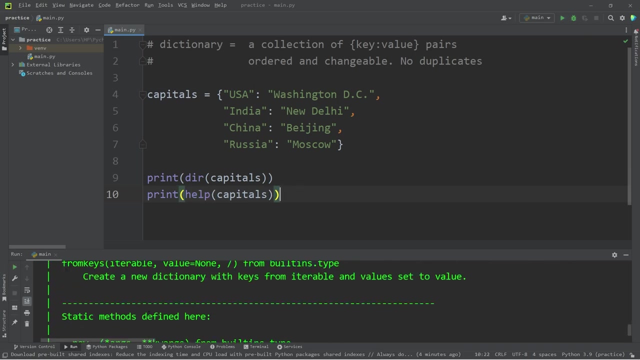 Here's all the different attributes and methods of a dictionary. If you would like an in-depth description of all these attributes and methods, you can use the help function. That's herp Help. There we go. So yeah, that's just a reminder. All right, let's cover a few of the methods. 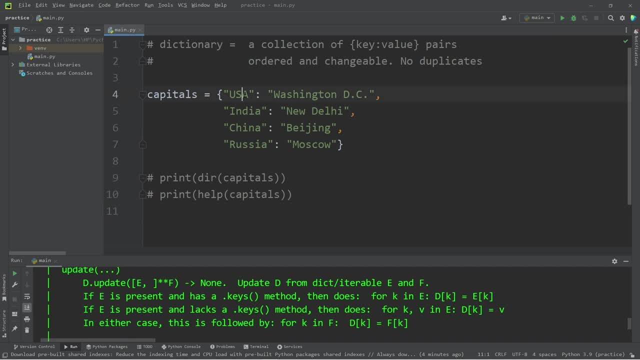 To get one of the values from a dictionary. you would get the key Type, the name of the dictionary: Capitalsget. Let's get the capital of the USA, Then we'll print it. The value associated with this key, the USA, is Washington DC. 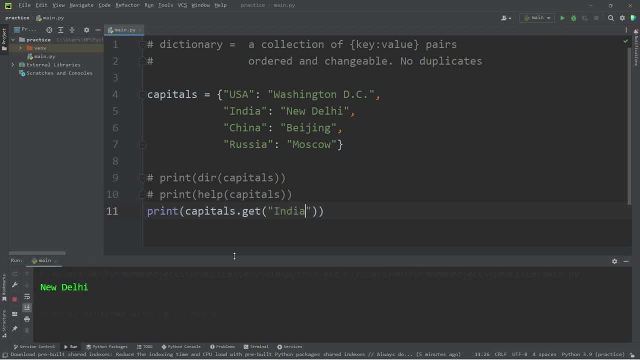 If I picked a different country, like India, well then we would get that associated value, which is New Delhi. Another thing: if Python doesn't find a key, this is what will be returned. Let's get Japan, which is not in our dictionary, This method. 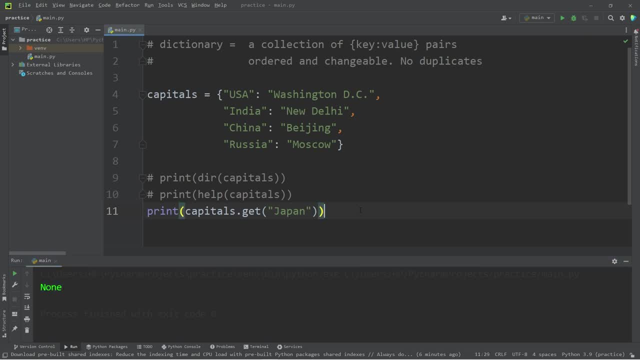 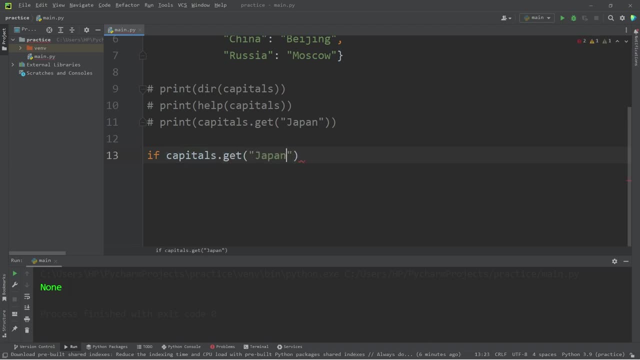 would return none. We can use this within an if statement. If capitalsget Japan, if a value is returned, then we will print that capital EXISTS. Else, we will print that capital DOESN'T EXIST. So Japan is not in our dictionary. that. 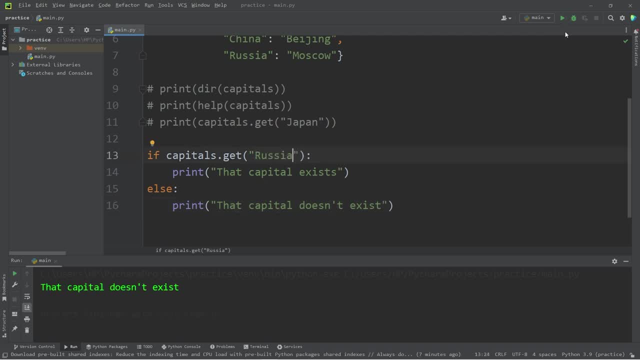 capital DOESN'T EXIST, but Russia's. that capital DOES EXIST. So Japan is這邊. Japan doesn't exist, But in our dictionary not Japan. So it'sاد confinement is not Japan doesn't. That's how to check to see if a key is within our dictionary. 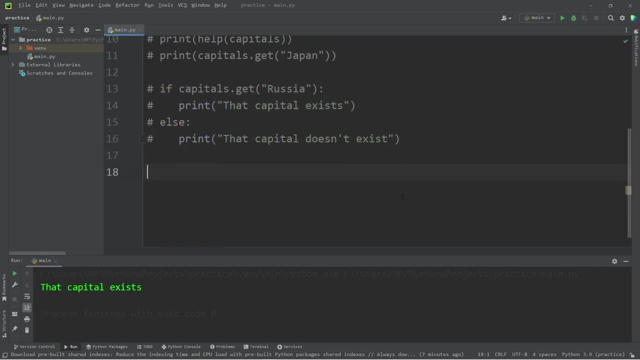 You can use the get method. Alright, moving on, Let's update our dictionary: capitalsupdate. So, within a set of curly braces, I will add a key, then a value: Germany, Followed by Berlin. Then let's print our dictionary. I'll use a print statement. 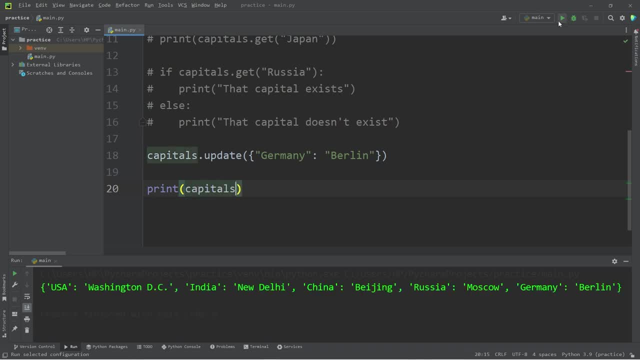 print capitals. Yeah, and there's Germany right there. Using the update method, we can insert a new key value pair or update an existing key value pair. Let's also change one of the existing values With our key, USA. let's update the capital to be Detroit. 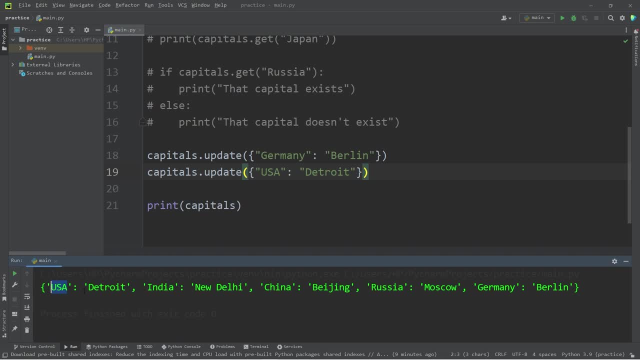 Yeah, see, the value has been updated. The capital of the USA is now Detroit, Michigan. To remove a key value, you can use the pop method, Then pass in a key. Let's remove China. China no longer exists within our dictionary. 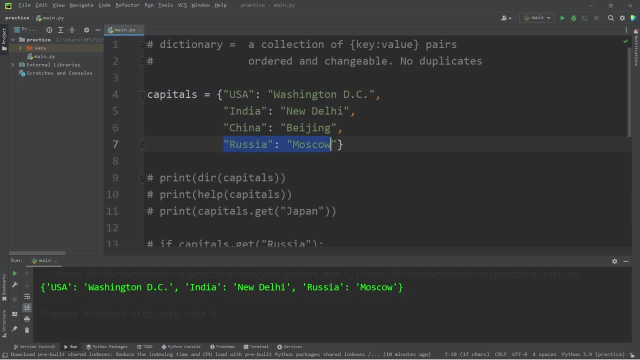 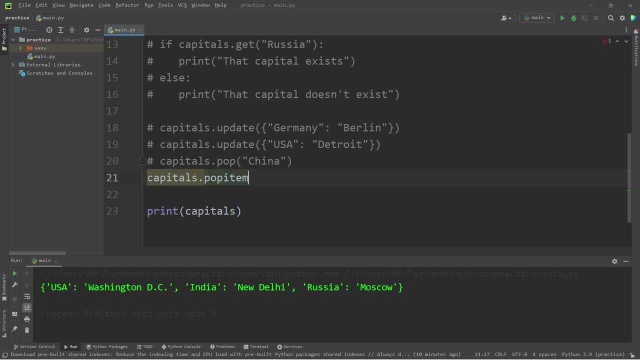 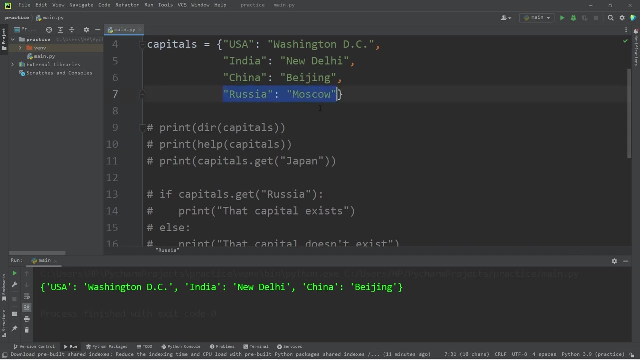 It's gone. You can remove the latest key value pair within a dictionary by using the pop item method: capitalspopitem. With pop item, you don't need to pass in a key. Pop item will remove the latest key value pair that was inserted. 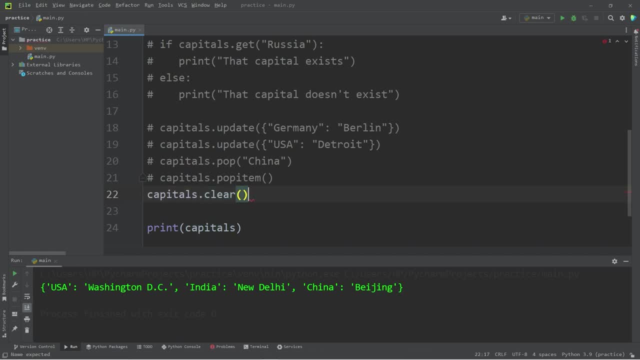 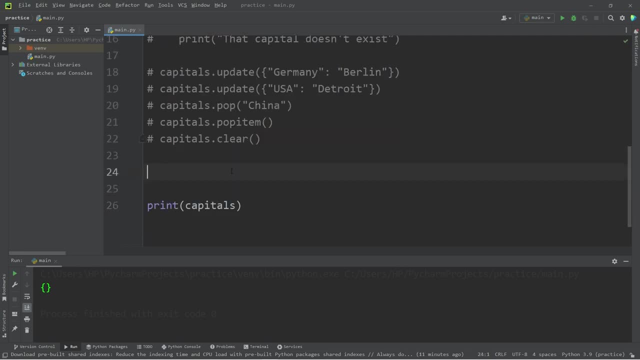 Then we have clear capitalsclear. That will clear the dictionary. It's pretty self-explanatory. The next few methods are a little tricky to explain. To get all of the keys within the dictionary but not the values, there is a keys method. 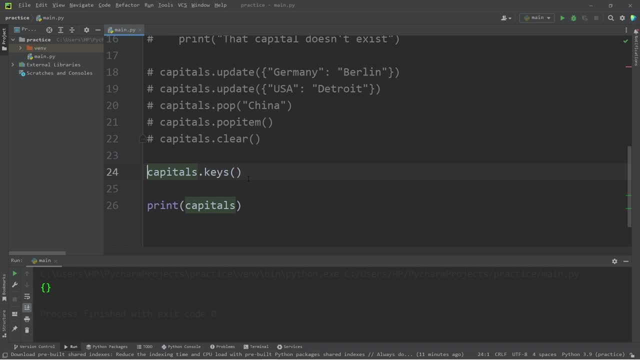 capitalskeys. I think I'm going to insert this within a variable. keys equals capitals, dot keys. Let's see what happens when we print this. The keys method will return all of the keys within our dictionary. Technically, keys is an object which resembles a list. 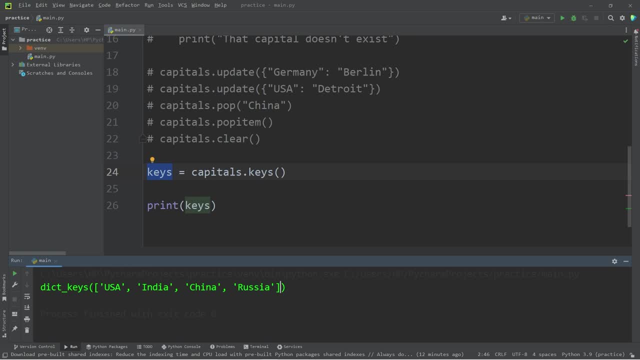 I haven't discussed object-oriented programming yet. This is a little bit above our level. If you ever need the keys in a dictionary, you can use the keys method. One use is that we can use that within a for loop. They're iterable. 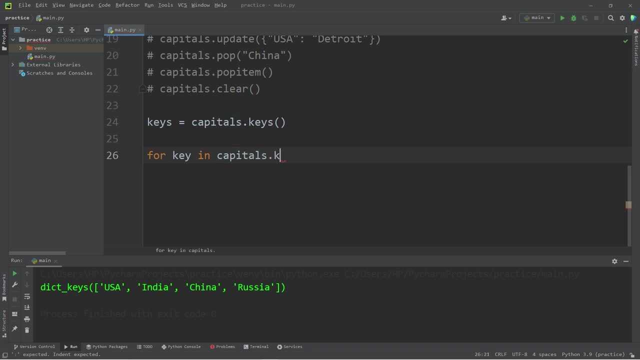 for every key in capitals, dot keys method. Let's print every key. If, at any time, you need to iterate over all the keys, you can use a for loop to iterate over every key that is returned from the keys method of your dictionary. There's also the values method.